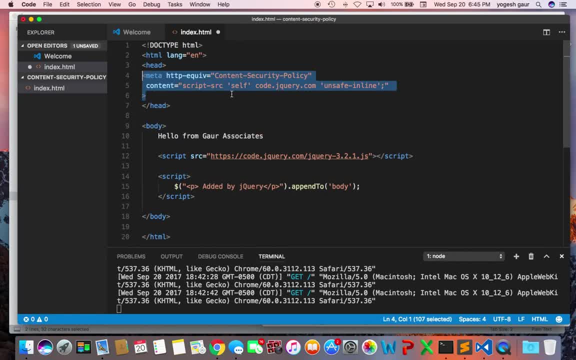 one particular way. So the one easy way to do is through what is called a meta tag, And in a meta tag you can add in the HTML itself And you can say: HTTP equivalent is equal to content security policy, And then you define your content to be something, something. So let's say, typically, what you want to do is you want to essentially, 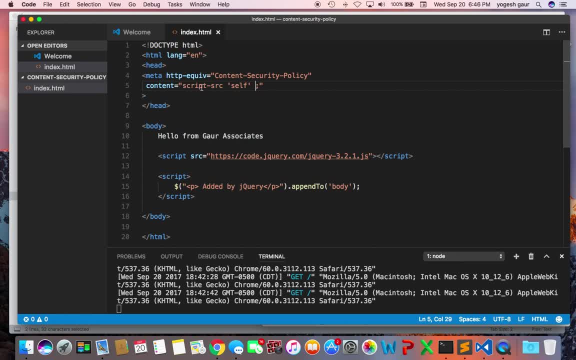 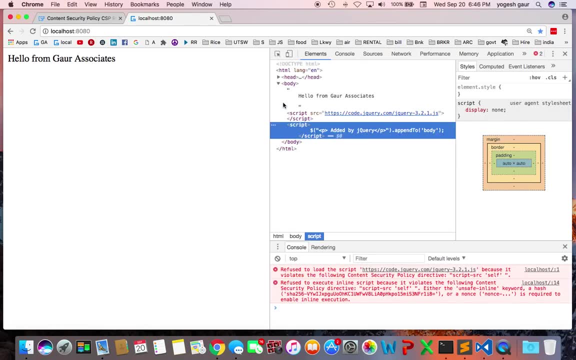 allow scripts only from your website. So you could just say: script source is yourself. And if you did that, let's see what happens if I reload this page. See, you can see this jQuery is not getting, the script is not getting loaded And this is how you could use the content security policy. And it is actually telling you in Chrome because it only has the script source self, And that's the reason why it is not working. So let's just go back to the 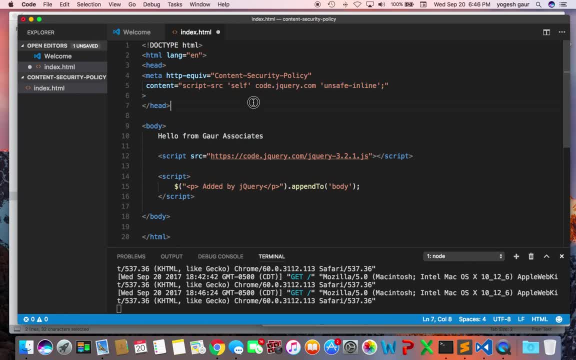 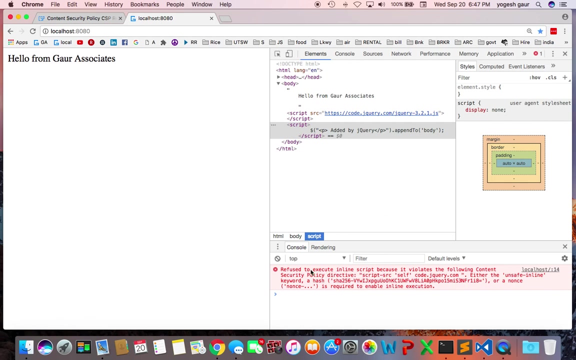 back there and put that back in again. So the next line I'm going to show you is if we can just say that we want to be able to download scripts from the same website and also from codejQuerycom, which is where I'm getting this script from, And if I just did that, I should get a basically a different error, because it says it was able to download the script but it cannot execute this portion of the code which is inline. 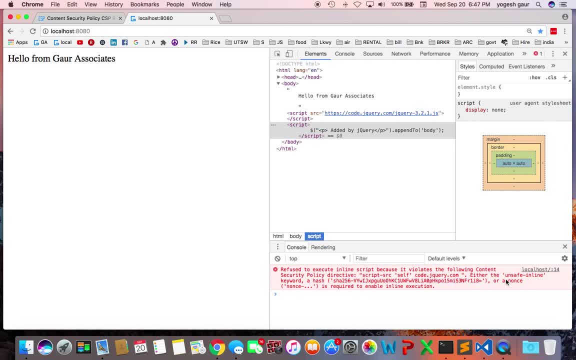 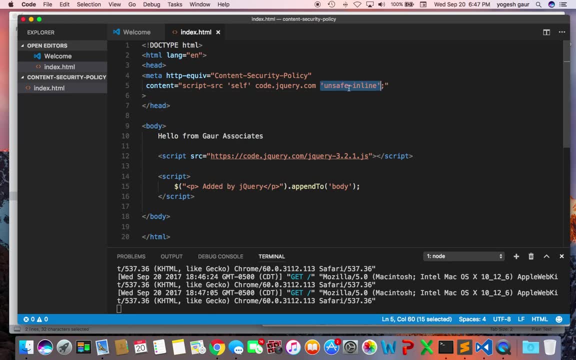 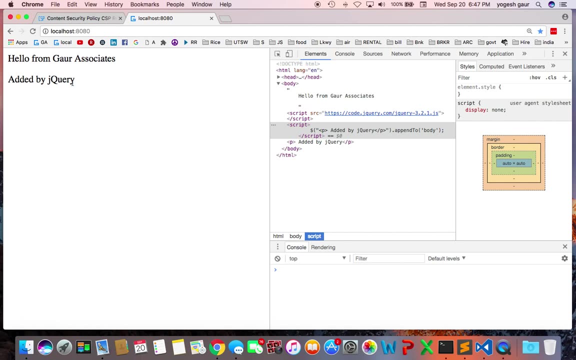 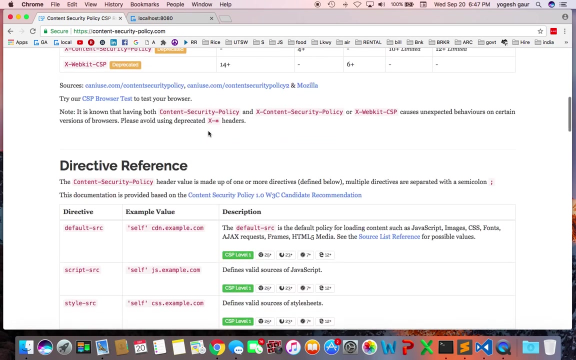 script, And the reason is I didn't add unsafe inline. So if I add unsafe inline, I would be able to execute this inline JavaScript and be able to see the result. And here you can see now it all works. So, essentially, what you want to look for is in the content security policy, And right now I'm just using this script source directive, but they do have directives for default source. 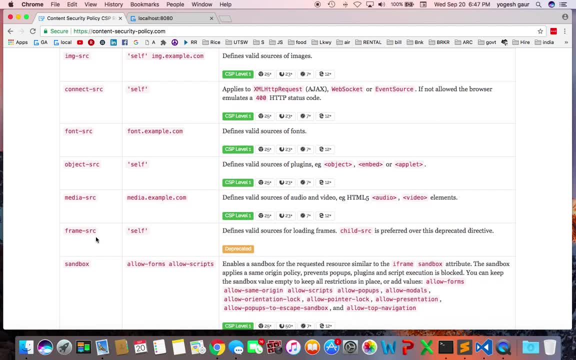 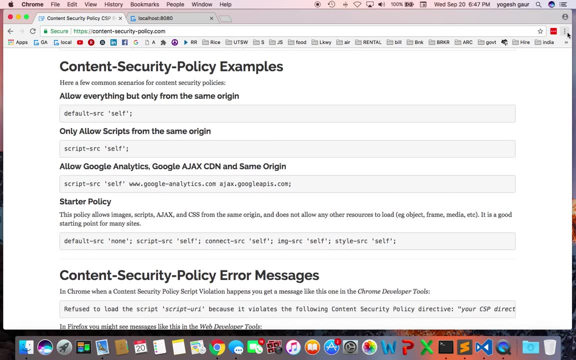 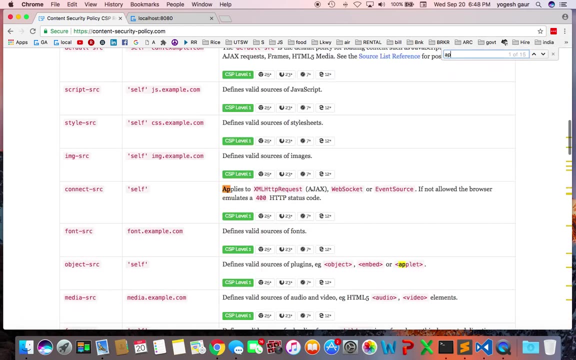 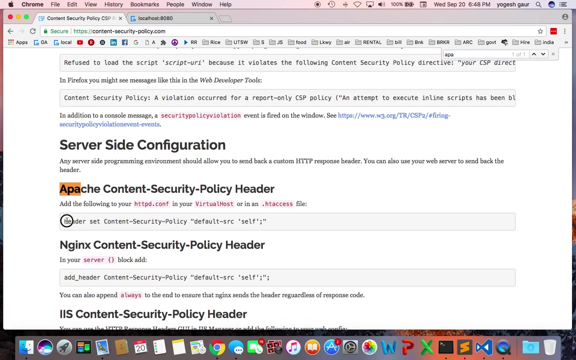 styling, imaging and fonts and all kinds of different stuff, And you can actually add this in the header tags as well, And it actually, I think, might show you here how to do it on the Apache, but I'm not sure. Let's see. Yeah, so it is actually telling you how to add content security policy header on the Apache itself and some other servers. So thank you for watching this short screencast And